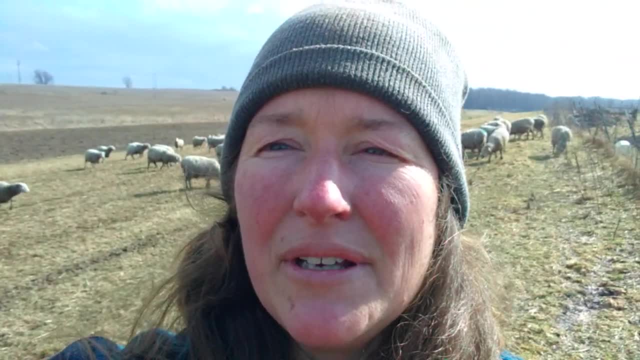 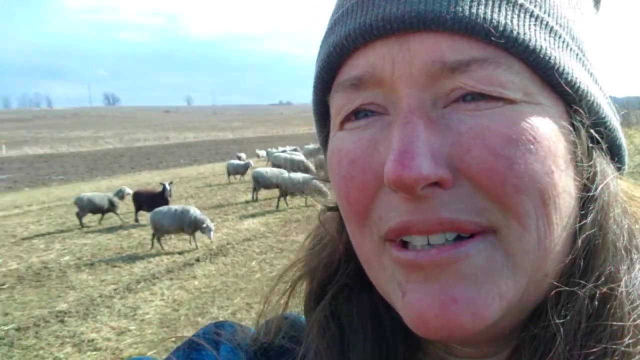 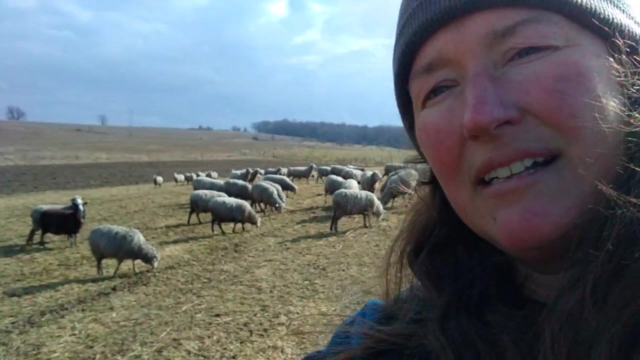 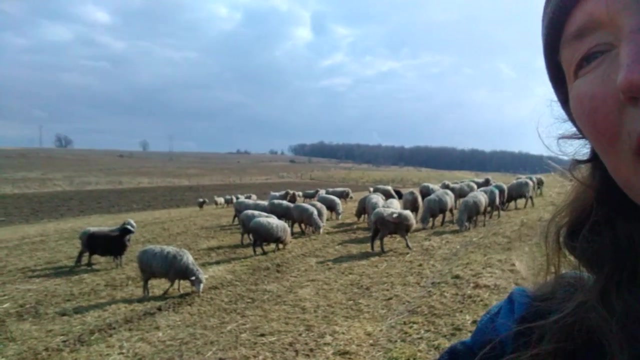 there's some ewe lambs in the field behind me and notice I called them ewe lambs. All these gals- let's see if I can turn this around. all these gals are just about well, they'd be 10 months old. They'll be starting to turn a year old in May and it's March 3rd today. 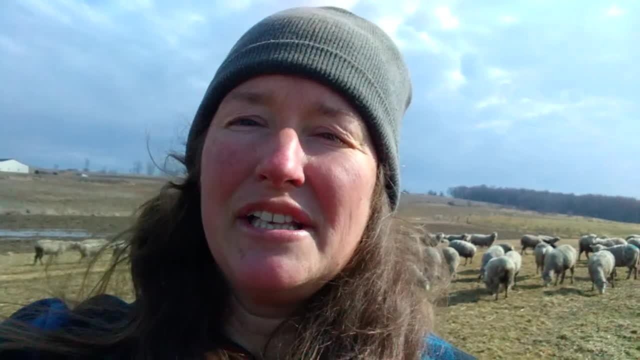 So, despite the fact that they're pretty big and actually these are brad ewe lambs, they're all ewe lambs. they're all ewe lambs. So, despite the fact that they're pretty big and actually these are brad ewe lambs, 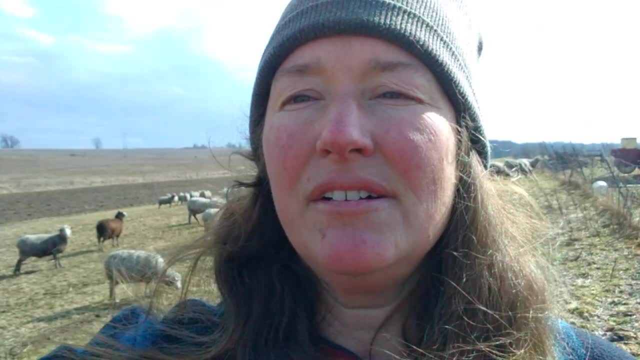 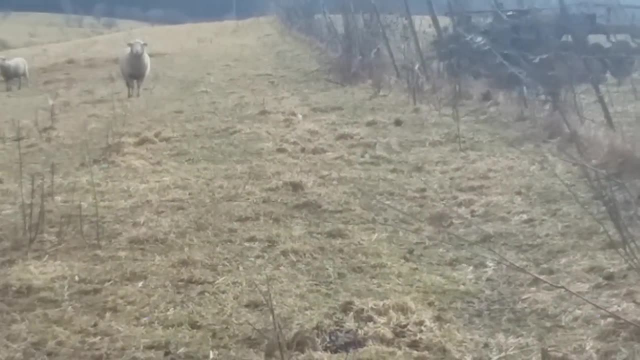 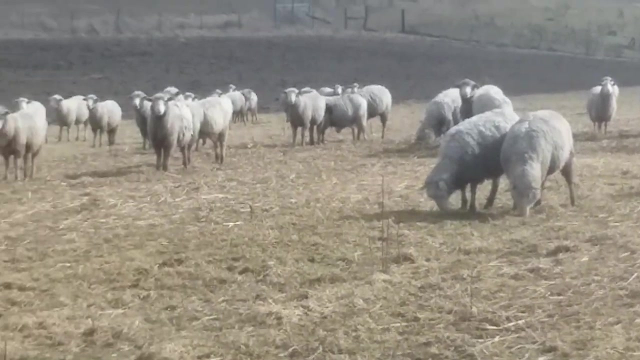 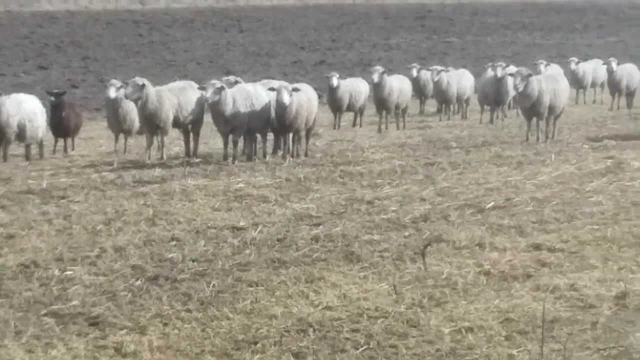 going to be moms this spring. they are still in the world of sheep called lambs. The guy furthest to the right kind of looking at me chewing his cud, that's the ram. Everybody else out here is a lamb. These are all lambs that were born. 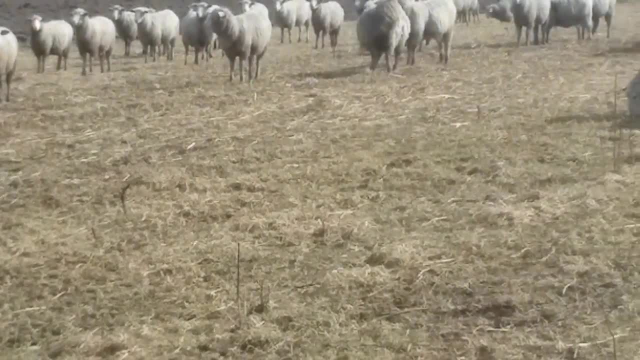 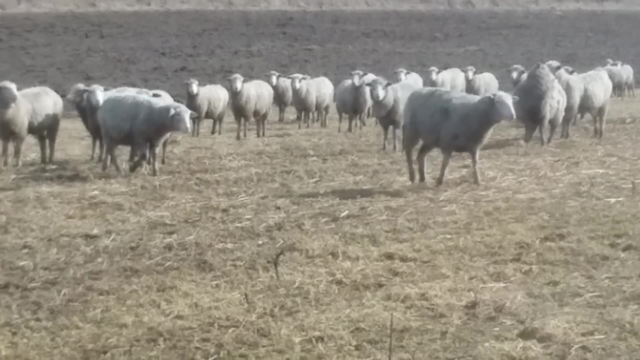 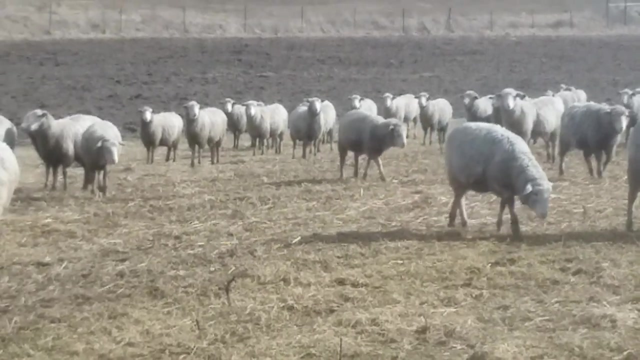 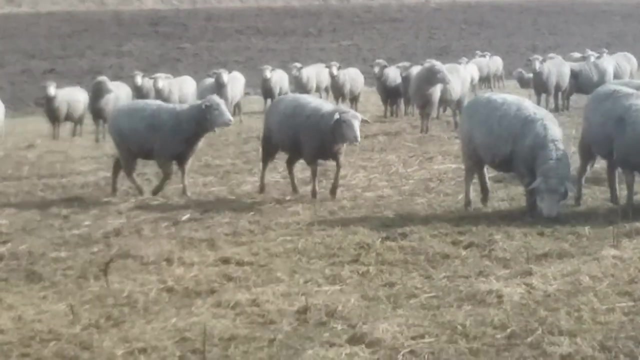 here this past year. most of them were born in May. But as far as what to officially call them, these gals are near full grown and are still called lambs. But as far as what to officially call them, these gals are near full grown and are still called lambs. 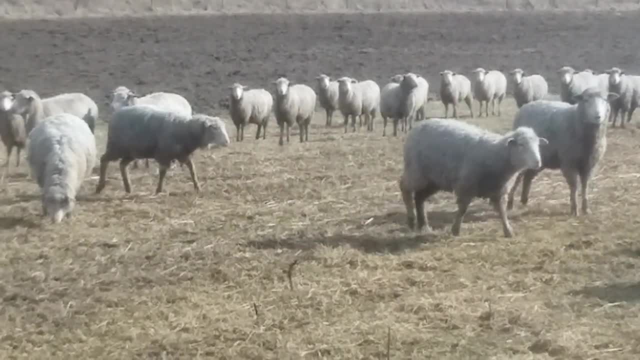 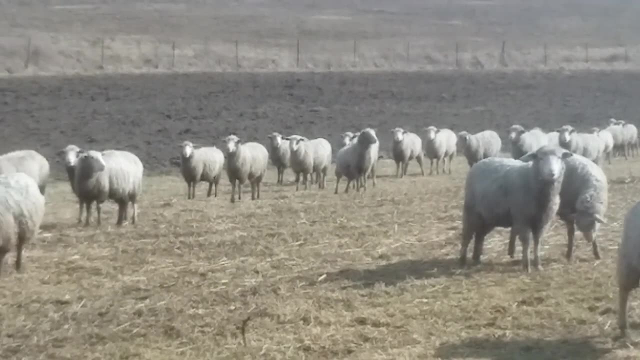 But as far as what to officially call them, these gals are near full grown and are still called lambs. And to these I just really wanna say: in the어야 wait, Once they reach their first birthday, they'll still be called lambs. 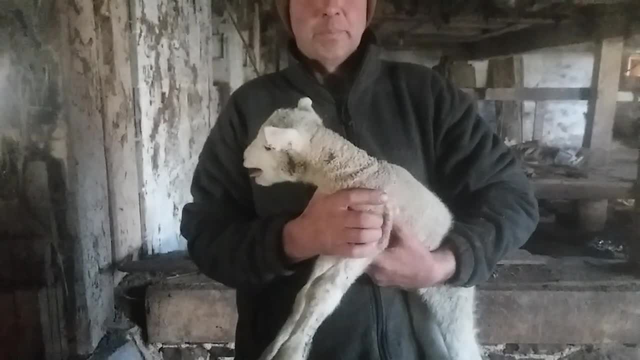 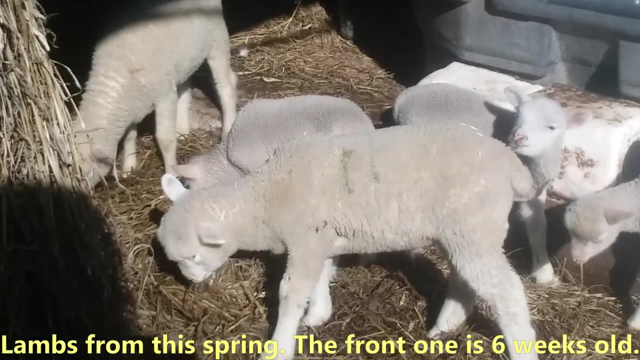 This guy's a week old. and he's also a lamb. aaaaah ahhhhh speeding going in speeding going in speeding going in moving moving leaving 人 UVU moving using the air � music playing. inspiration for music playing in the background whileiend toward the air freedom. 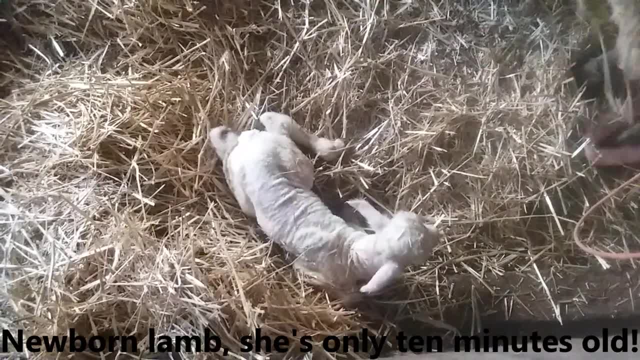 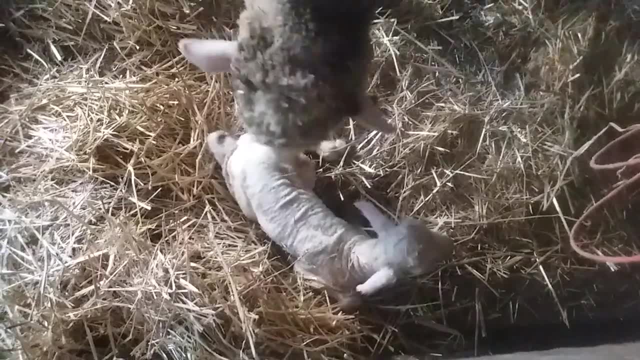 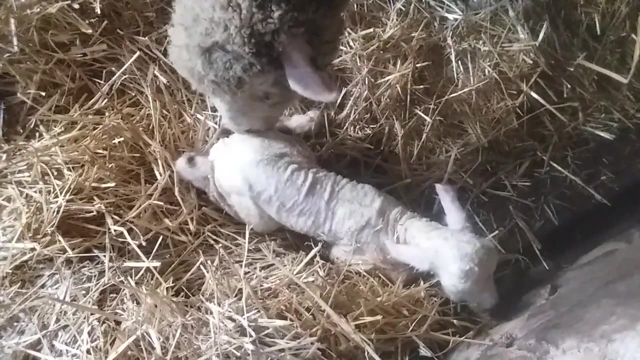 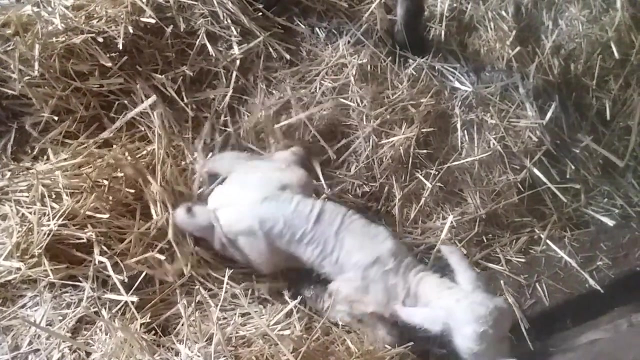 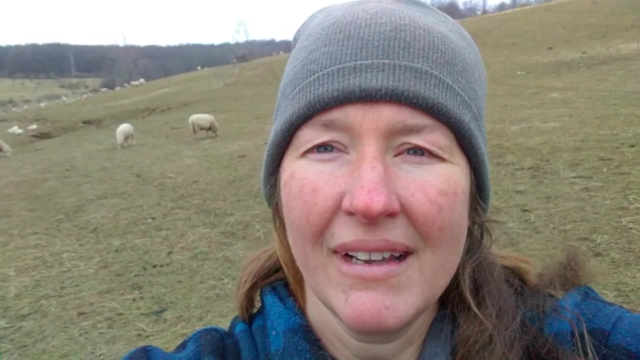 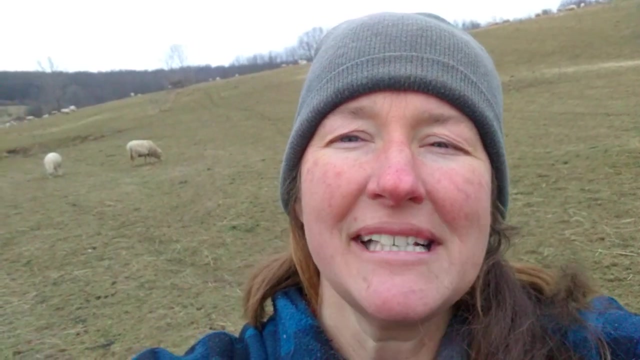 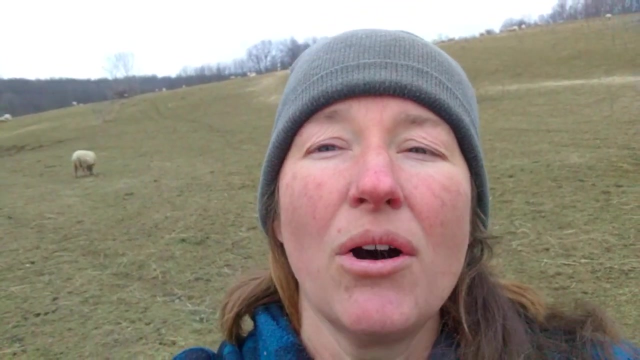 wrinkles. Semons song playing: Uhhh, Uhhh, Uhhh, Uhhh, Uhhh, Uhhh. now we're out with the main flock of sheep. notice: i said sheep, not lambs, and the reason i said sheep is because everybody out here is going to be too shortly or older, so the youngest 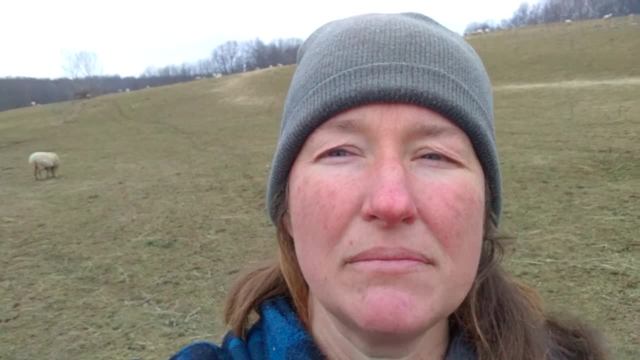 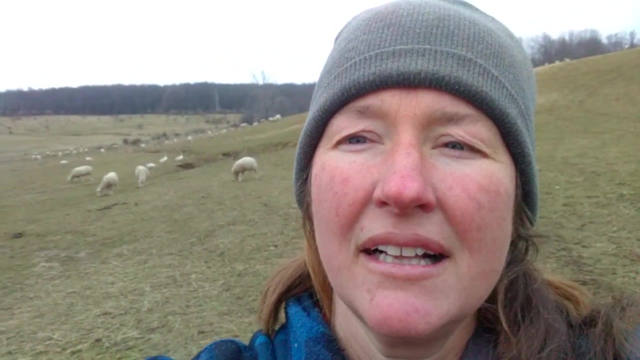 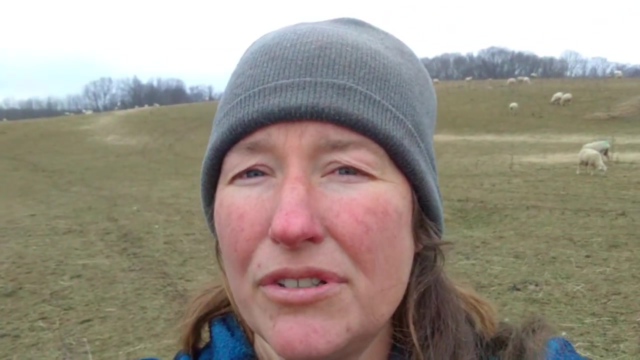 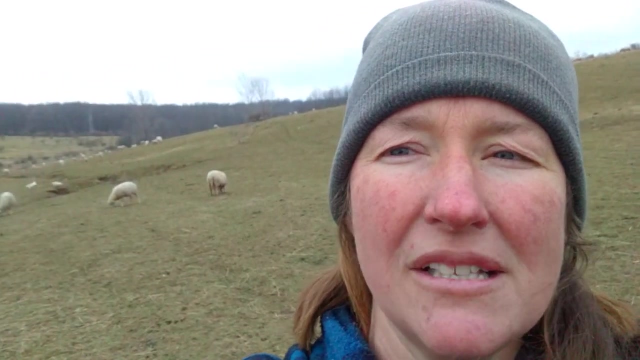 out here will be turning two, probably in may, and it's early march right now, so we'll look around a little. you can see there's some geese out here too. so this is the flock of adult sheep. no lambs out here yet. the lambs will be born in a couple months, starting in may. 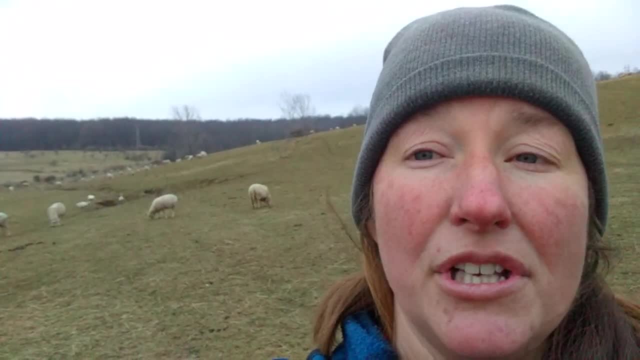 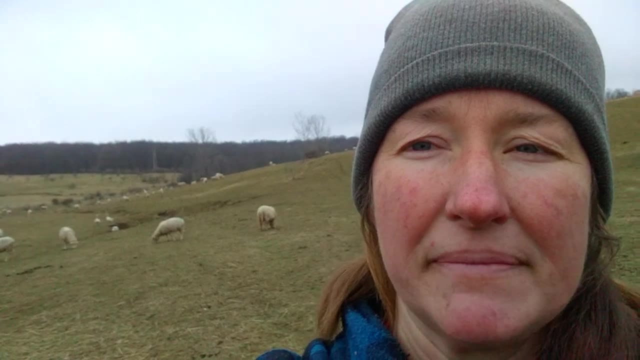 so these sheep would actually be called sheep because of their age, since everybody out here is going to be turning two because they're older, so these sheep would actually be called sheep because of their age. so these sheep would actually be called sheep because of their age. here is over one, They're all referred to as sheep And it's starting to rain a little. 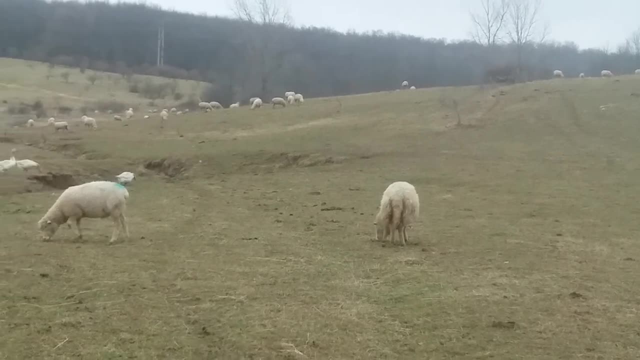 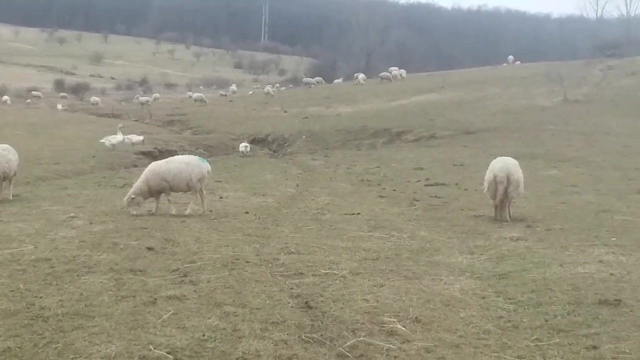 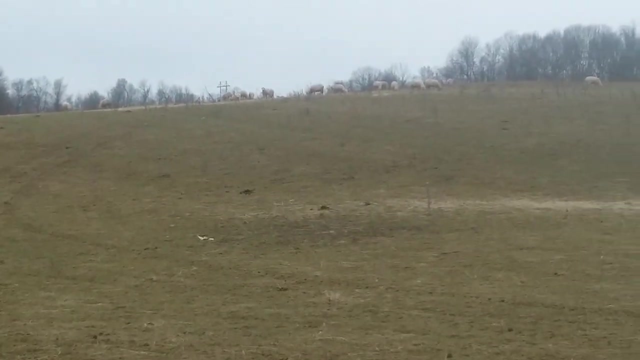 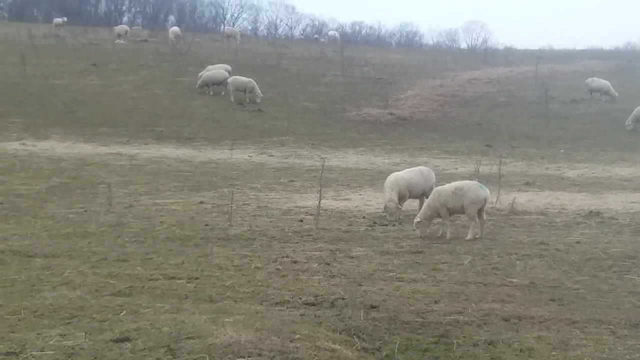 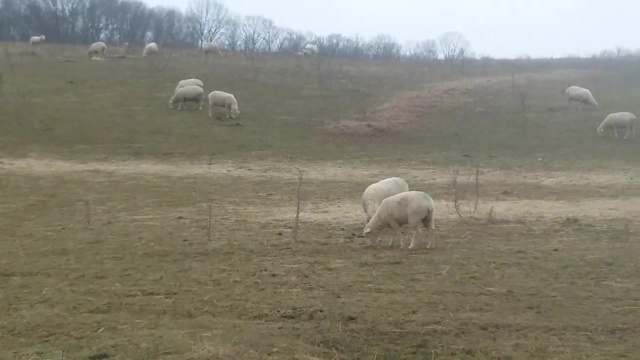 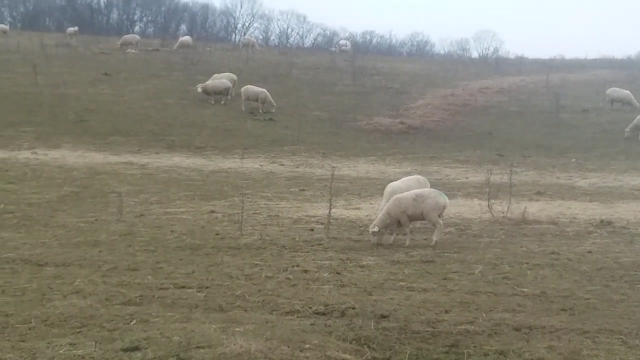 bit. Not too surprising. That's pretty normal for us this year. There's a few more up there on the hill, A couple a little bit closer here. Like I said, everybody out here is an adult. There are a few rams, but everybody is just shy of being two or older. 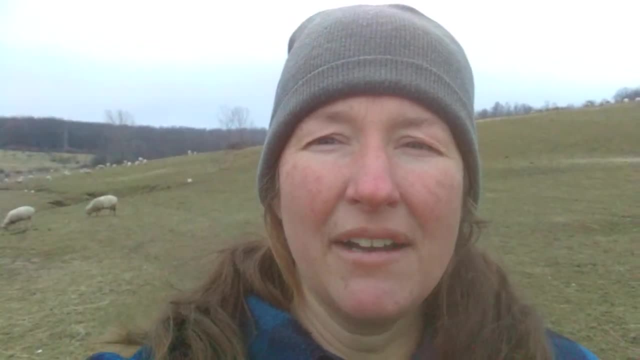 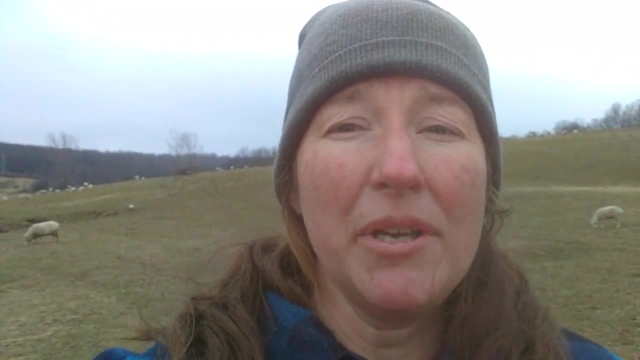 So, to sum it up, going from a lamb to a sheep is kind of like you when you turn 18, at least in the United States. The week before your 18th birthday, you were a kid. Then, once you have your 18th, 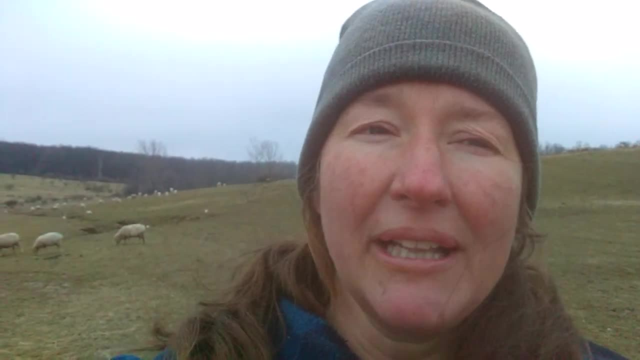 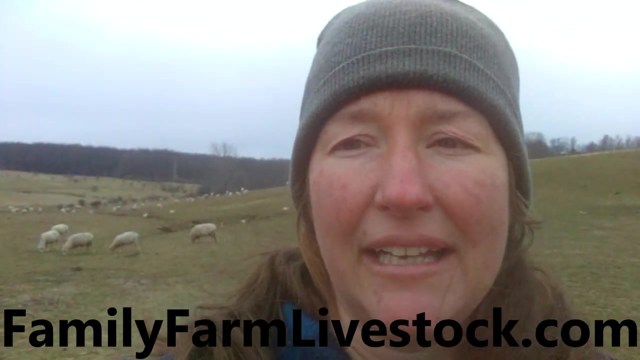 birthday. now, all of a sudden you're an adult, But really there's just a few days difference there. So we have to draw the line somewhere, And with sheep versus lamb it's at a year old.